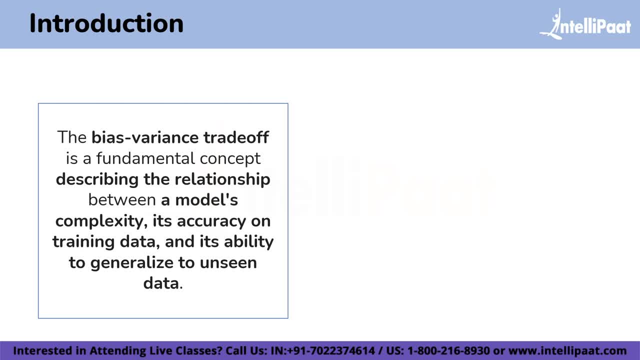 bias and various trade-off before we start with the basics. So the bias and various trade-off is basically a fundamental concept which describes the relationship between a model's complexity, its accuracy on training data and its ability to generalize to any unseen data. And this 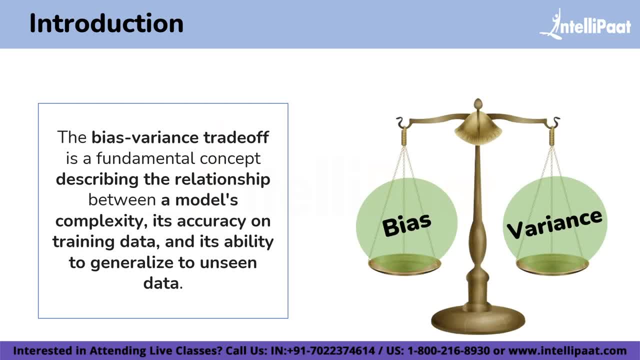 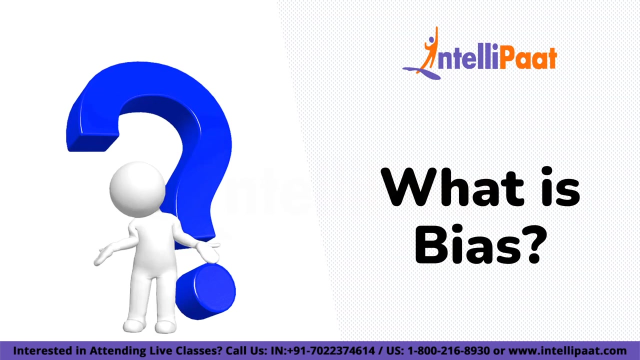 is essentially a balancing action. Ok, let's begin with the basics. So when we come back to our machine learning model, we can see that bias and variance are two sources of error. that is, bias and variance. So generally, these are the two sources of error that affect our model's predictions. 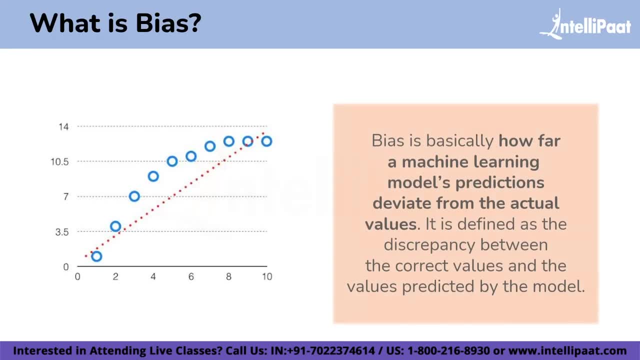 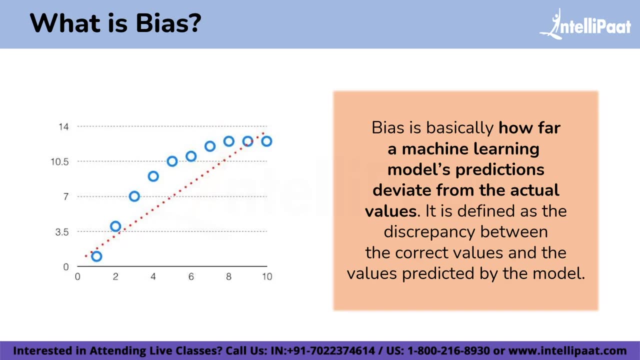 Right Now, let's begin with the basics and we'll see how they make a difference to our machine learning model. So let's first start with what is bias- the correct value that we are trying to predict, like as you can see in this graph. 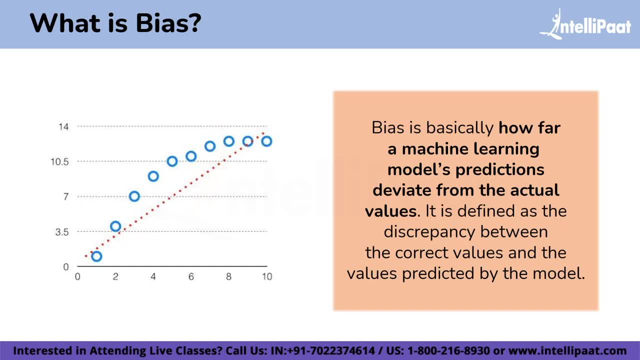 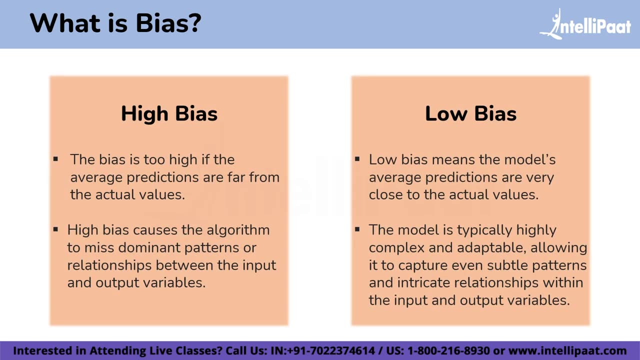 how far does a machine learning models predictions deviate from the actual values? so this is defined as the disparity between the correct values and the values predicted by our model and, as if you are talking about bias, there are two types in it: high bias and low bias. so high bias makes a strong assumption. 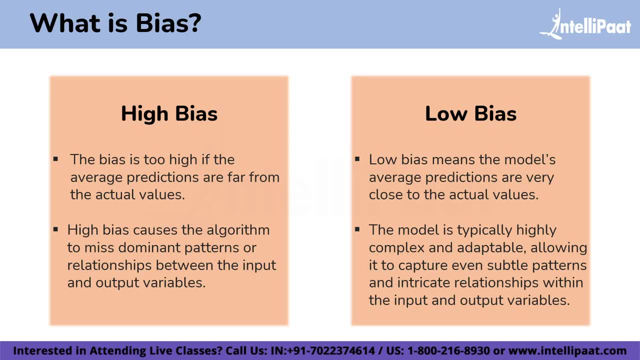 about the data over simplifying it and ignoring the complex patterns that were present in the data. whereas low bias makes the fewer assumption about the data, allowing for flexibility and can capture a complicated patterns in the data, and that's why it is recommended that an algorithm should always be low. 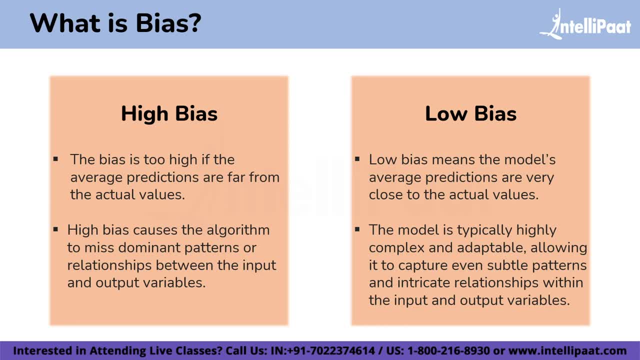 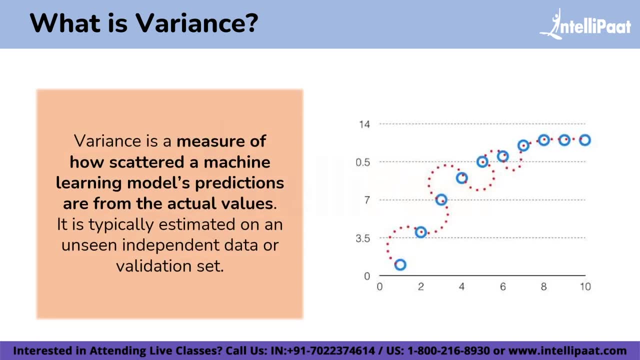 bias to avoid the problem of under fitting. now let's look into what is variance. variance is basically the variability of models predictions for a given data point or a value that tells us the spread of our data. so, as you can see in this graph how scattered models predictions are from the actual values, 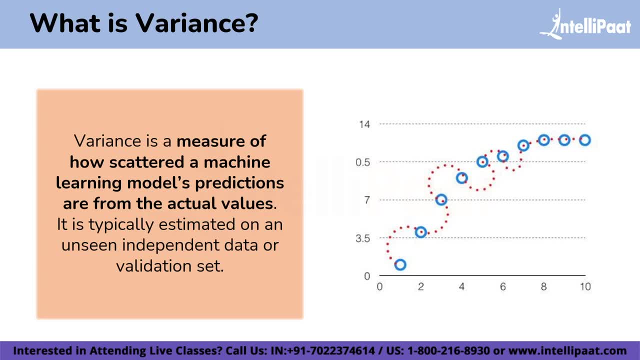 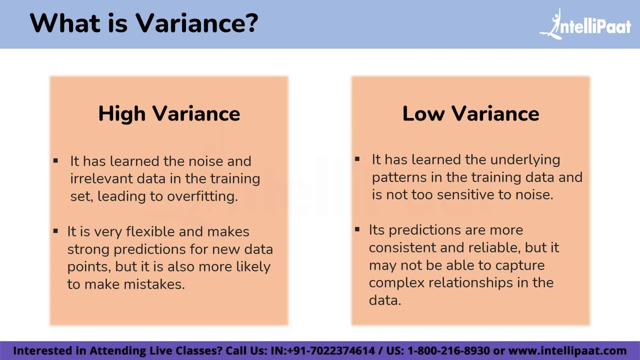 and it is typically estimated on unseen, independent or validation data sets only. and if you are talking about variance, here are also. there are two types in it: high variance and then sometimes low variance goes on top and it's based on the pattern changes. for example, it might be house run. it has three variables like radius and surface. 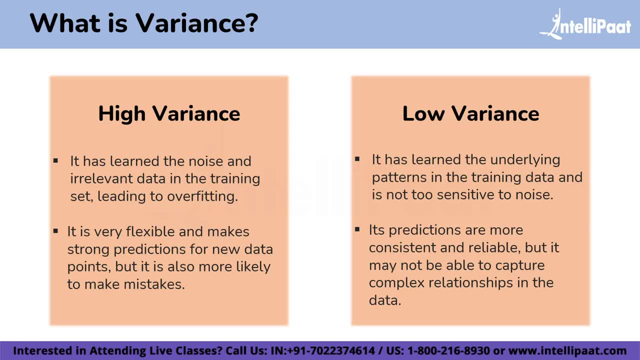 the opposite of those variables are very popular about the right, of course. so let's start off with the average here. if we say we had some un��고able sheets of the right different dimensions service, that means that they agree. let's assume I've produced some 64 by 5 houses and clearly that it typically 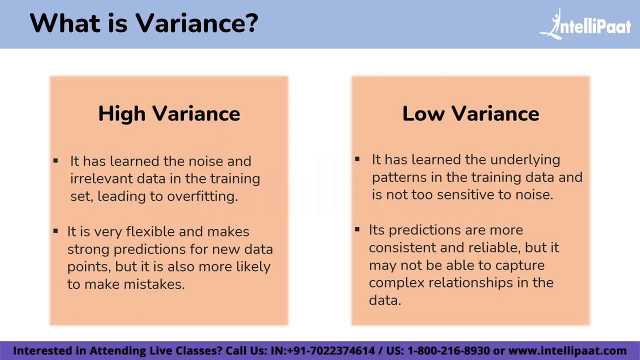 fits the sample. so at first look at the sample size and lowest one value and unload on the baseline is Lazarus will develop a total of some 200 areas or 100 hours. very simply, when we take the сравTraining of those tells us that the 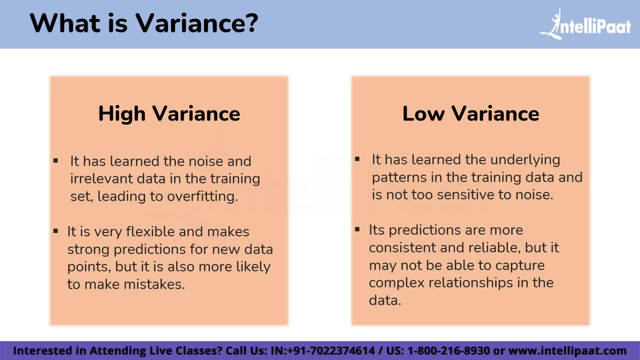 seen before. so, as a result, such models perform very well on training data, but have a high error rates on test data. and when a model is on high variance, it is said as overfitting of data. so don't worry, as we move forward in this video, we will try to understand both overfitting and 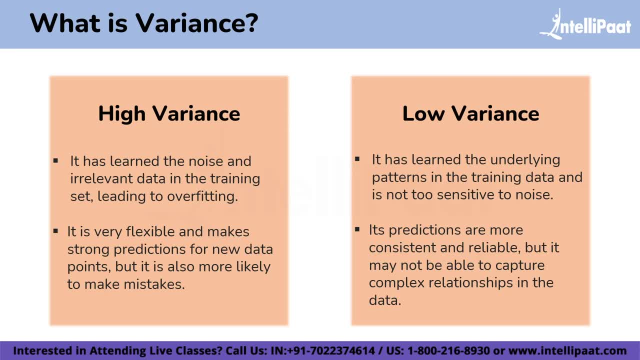 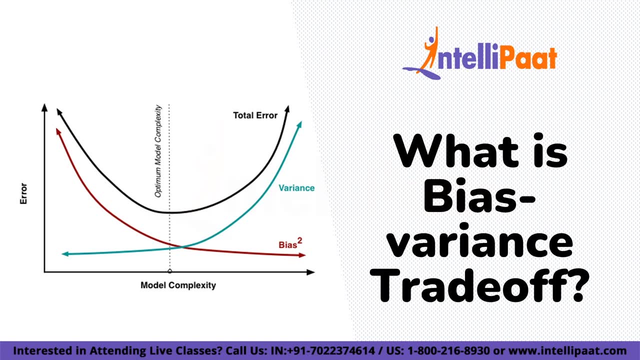 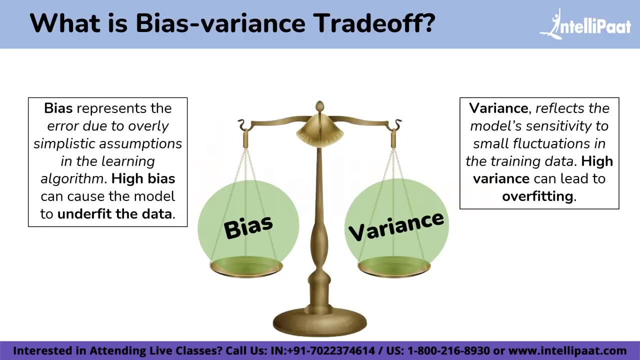 underfitting better with the help of examples and all. so make sure you stay tuned with us till the end. right now, let's jump on to our main agenda point, that is, what is bias and variance trade-off? okay, so, as i said in the introduction, the bias and variance trade-off is basically a fundamental 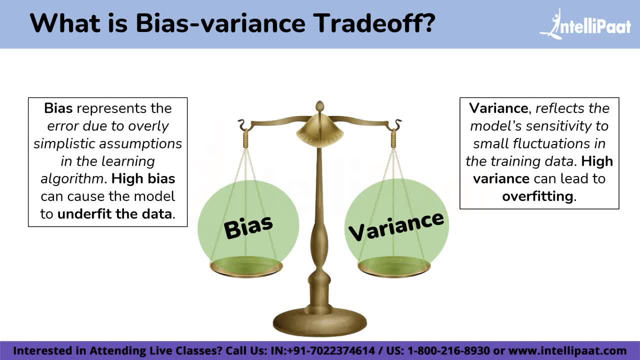 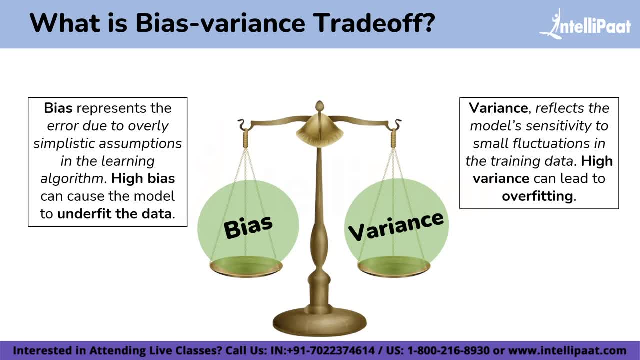 in the learning algorithm: high bias, which can cause the model to underfit the data and leading to poor performance on both training and unseen data. on the other hand, variance represents the model's sensitivity to small fluctuations in the training data. high variance can lead to overfitting. 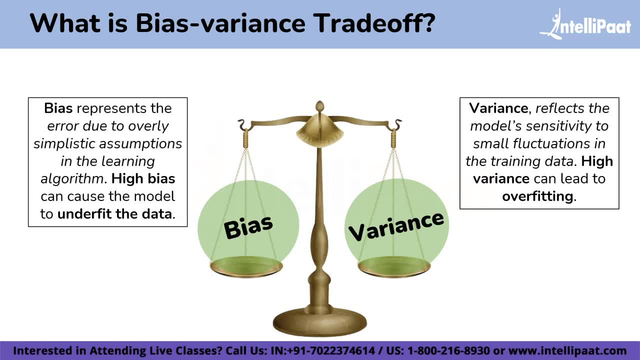 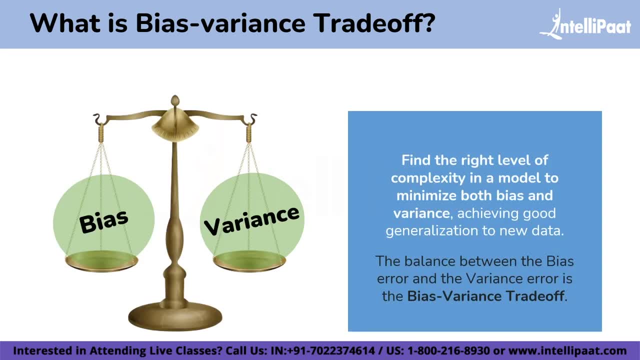 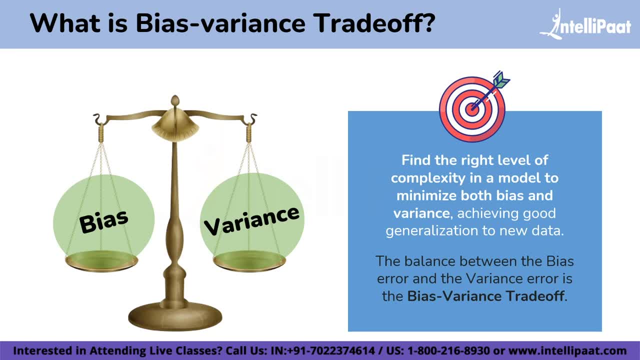 achieving a good generalization to new data, and balancing these two factors is essential for building models that perform well on variety of data sets. and if you see it in one sentence, then the balance between the bias error and the variance error is the bias variance trade-off. okay, now let's 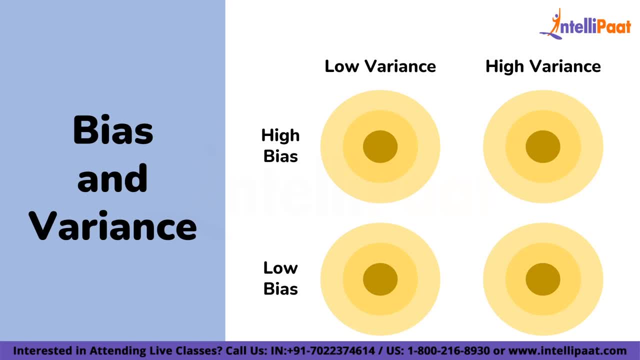 look into this bull's eye diagram which explains the trade-off better. so in the center- that is bull's eye- is the model result we want to achieve that perfectly predicts all the values correctly. and as we move away from that bull's eye, our model starts to make more and more wrong predictions. 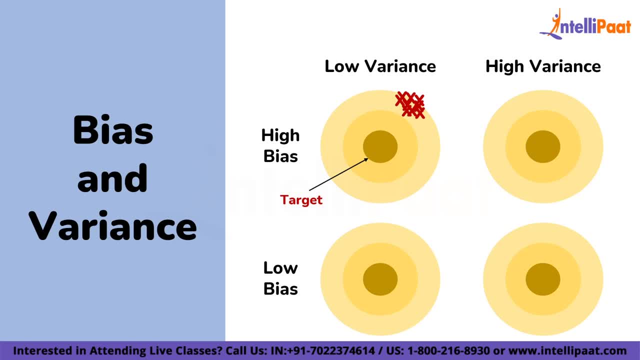 so here you can see four models: first, model with high bias and low variance. second model with high and high variance. third, model with low bias and low variance. and our fourth model with low bias and high variance. right, so here a model with low bias and high variance. that is this model. 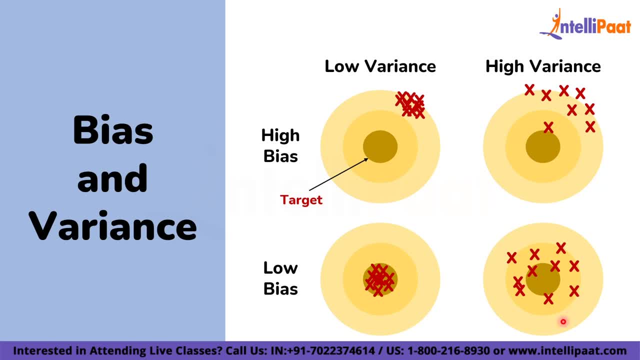 predicts points that are around the center generally but are pretty far away from each other, and a model with high bias and low variance. so in this model, as you can see, the points are pretty far away from the bull's eye, but since the variance is low, the predicted points are closer. 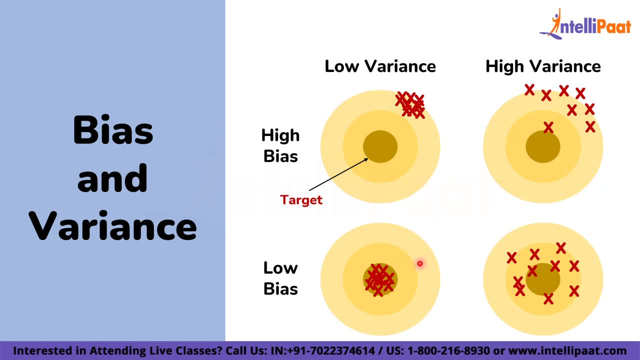 to each other. and if we look at this model with low bias and low variance that are around the central generally and also having a very minimum distance between them, is the balanced model that is neither overfitted nor underfitted. so here this model with the high bias is known as underfitting. 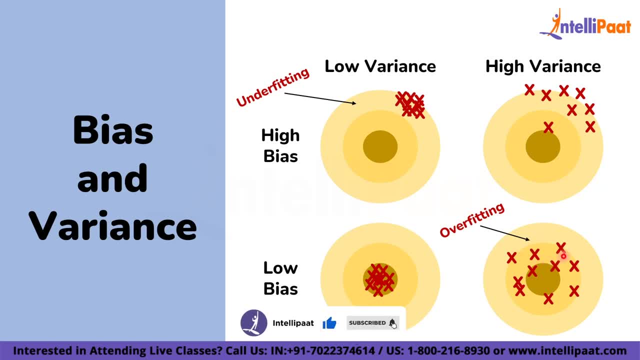 and the model with the high variance is known as the overfitted. and now, with these diagrams, you can clearly understand when a model is said to be underfitted, when it is said to be overfitted of the data and when it is said to be as the balanced right. 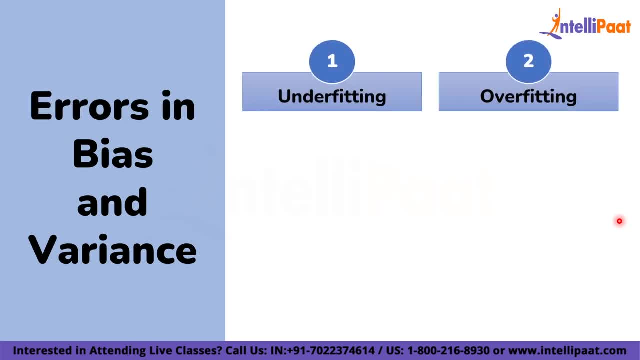 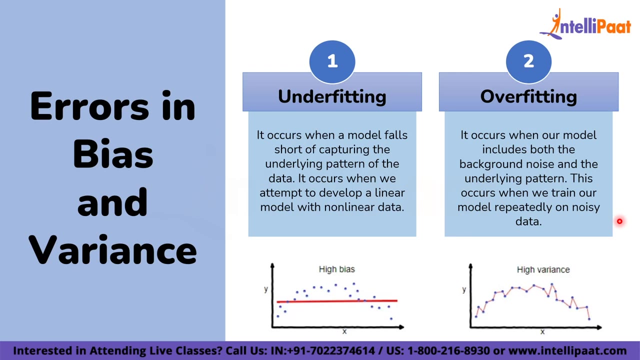 so these are the two errors in bias and variance that i talked before in this video. that is underfitting and overfitting. so underfitting basically happens when a model is unable to capture the underlying patterns of the data, and these models usually have a high bias and low variance, and it generally happens when we have 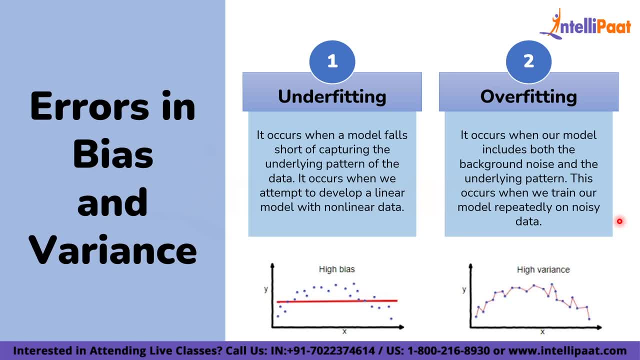 very less amount of data to build an accurate model, or when we try to build a linear model with a non-linear data. and if we talk about the overfitting, this happens when our model captures the noise along the underlying patterns in the data and it happens when we train our model a lot. 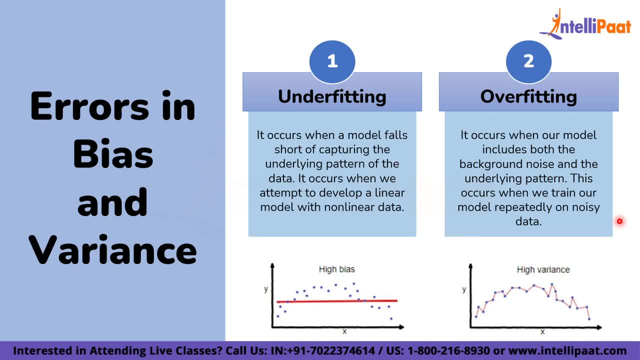 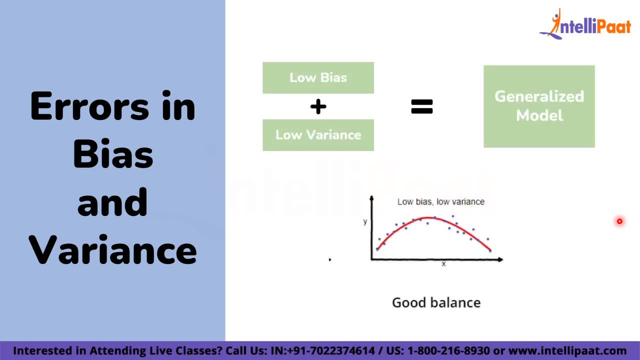 over noisy data sets. so these models have a low bias and high variance. so whenever there is a combination of low bias and low variance in a model, we called it a generalized model, and these are the models that give the best results to make any predictions. so we need to find the good balance without overfitting and 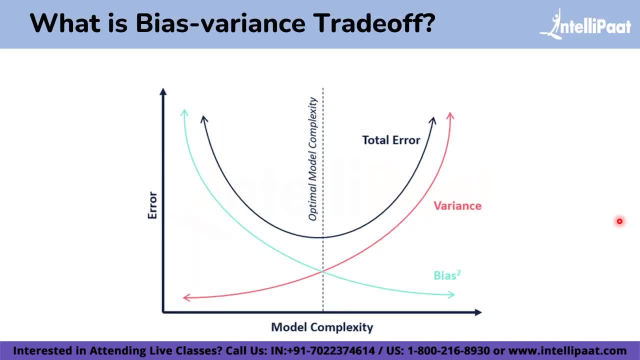 underfitting of the data. okay now, if i talk in terms of model complexity, we can use the following diagram to decide on the asset choice, on the FDE couple common ask mark setting об the optimal complexity of our model. so this graph is a classic illustration of bias and variance. 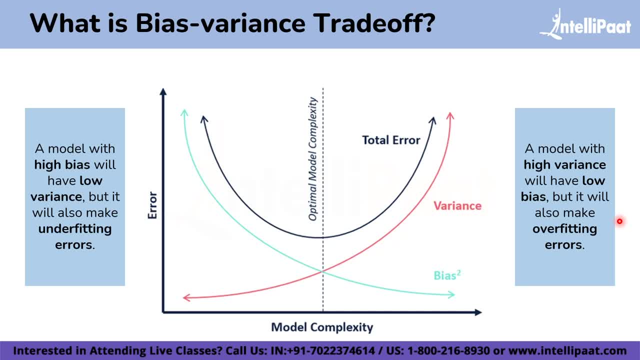 trade-off. so what this graph actually says is that in machine learning there is always a trade-off between bias and variance. like, a model with high bias will have a low variance, but it will also make an underfitting errors, whereas a model with high variance will have a low bias but will also. 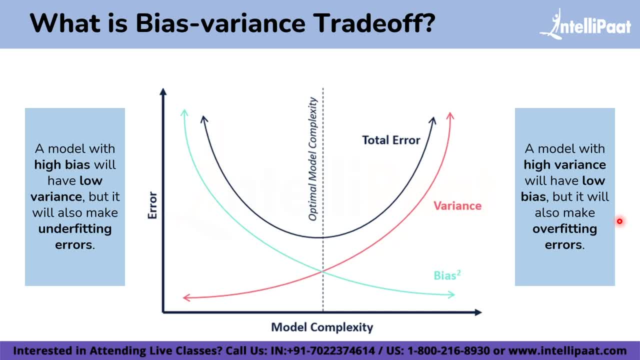 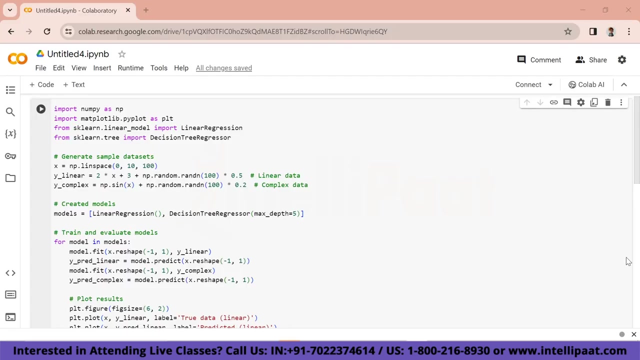 make overfitting. so the optimal model complexity is the point where the model has the lowest total error. so that points comes somewhere to this, as you can see optimal model complexity line here. so here that point will come where the model has the lowest total error. okay, so here i have this small python code snippet that help you understand this bias. 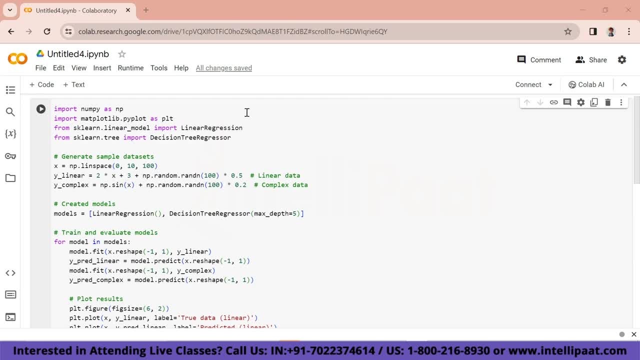 and variance trade-off. so here, first of all, i have implemented the model with high variance. so here i have this small python code snippet that help you understand this bias and variance trade-off. so here, first of all, i have implemented the model with all of the necessary libraries and prerequisites that i needed for this implementation. i will 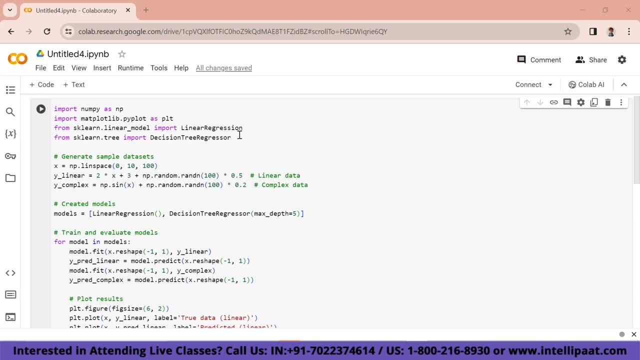 put it, number here- matplotlib and the two ml models, that is, a linear regression and a decision tree regression. here and after that, here i have created 100 evenly spaced points between 0 to 10 and then i have generalized linear and non-linear complex data with the noise in this section here. 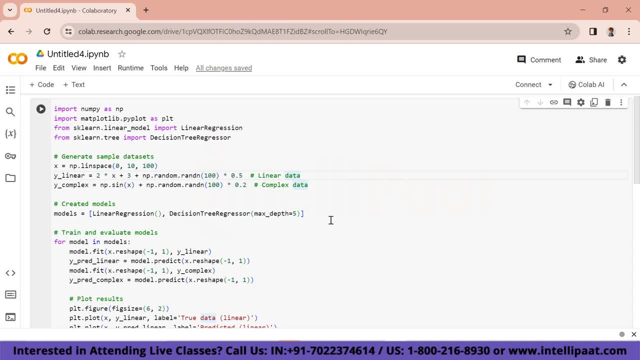 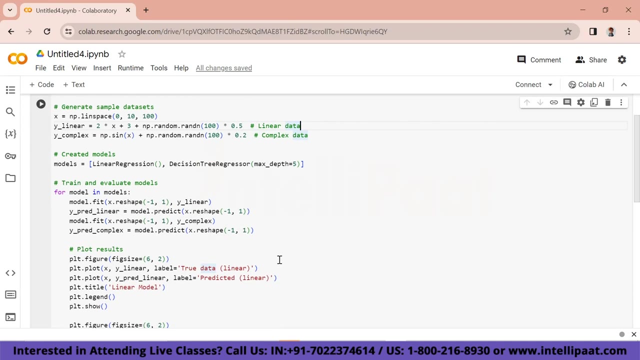 and after that, and after that I have created the list of our two models, that is, linear regression and a decision tree, and after that I have created here the list of our two models- that is, linear regression and a decision tree- regression- and after that here I have created a loop through each model. 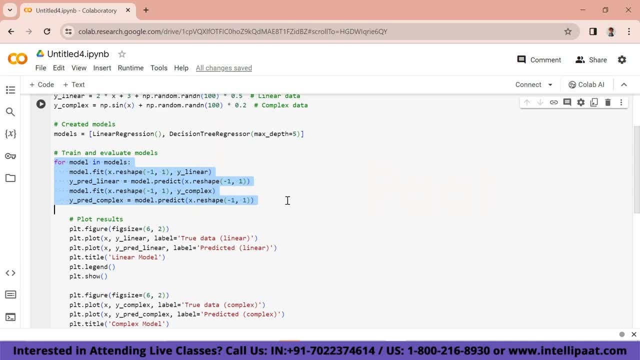 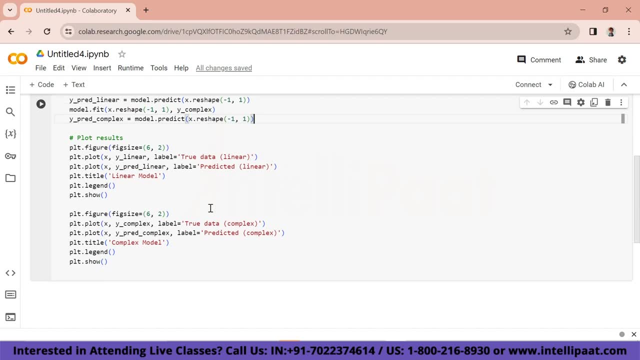 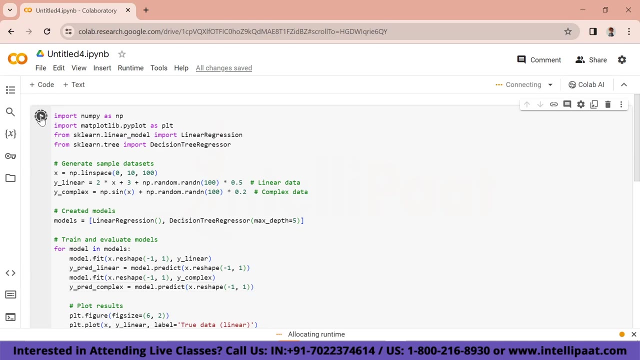 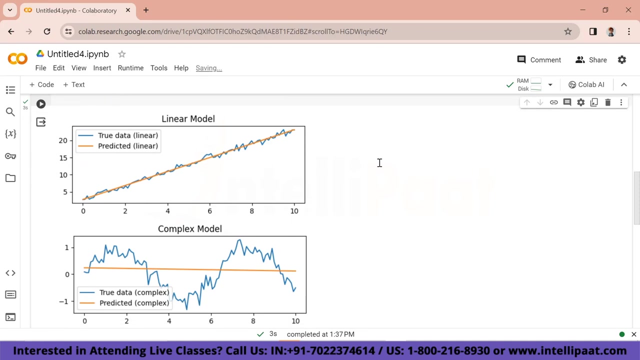 and I have trained, model and predicted both linear and complex data, and then, finally, I have plotted the result here for linear model and for the complex model here. So now let's run this code snippet and see the output for it. Okay, guys? so here in this initial graph, you can see how both the linear and complex models 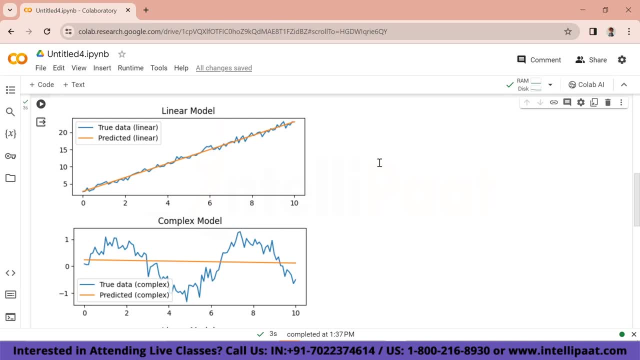 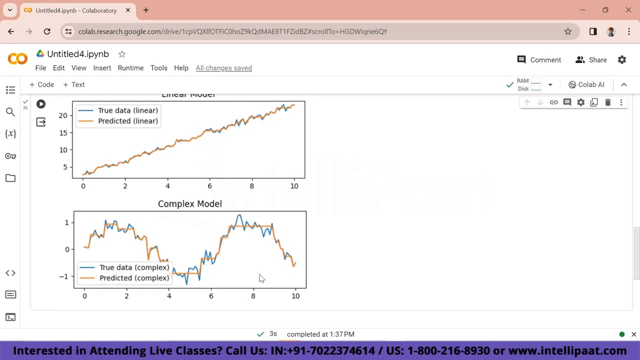 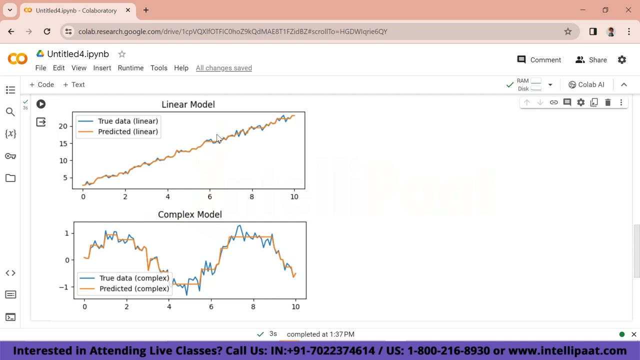 having a big difference in their true data and the predicted one. right You can see true data is in blue line and the predicted one in the orange. in both of these graph you can see a big difference in them, right. but in the second graph you can see how true data and predicted ones are balanced. here you can see both these lines. 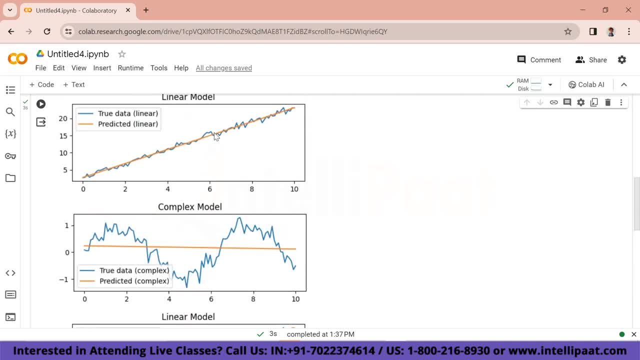 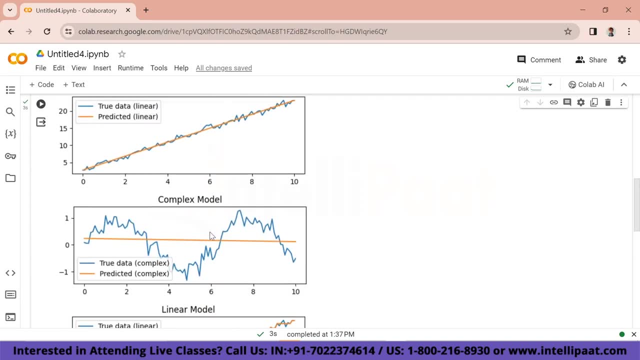 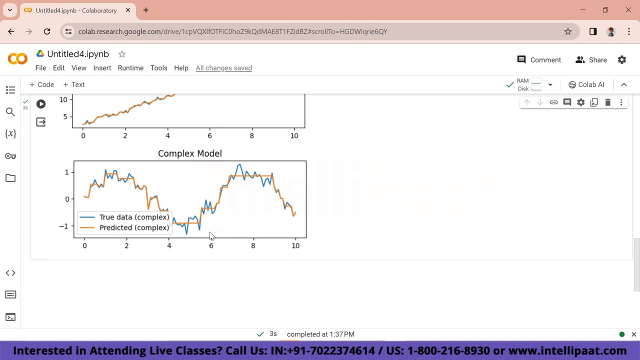 true data and predicted- are little balanced than the previous one. here and, in same as in complex model, you can see they are more balanced than the previous one, right? so that is basically the trade-off between buyers and variants. okay, now let us move forward and see how to reduce this trade-off. 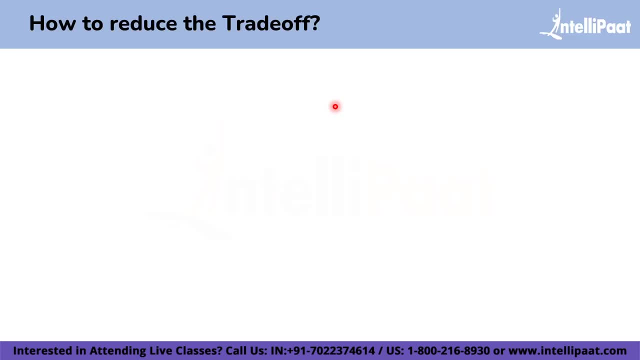 so there are several techniques that can help you reduce the trade-off between buyers and variants and help you improve your model's performance. so the first method is cross-validation. so in this method we split our data into multiple subsets and use some of them for training and some 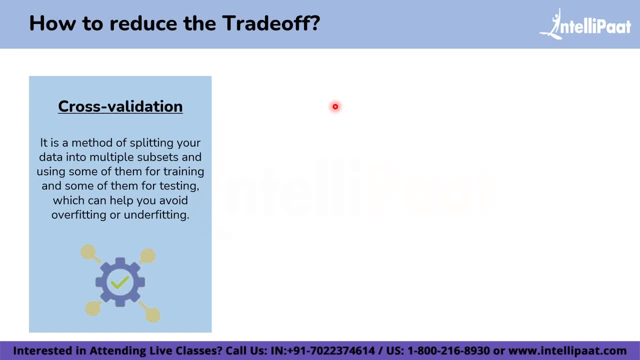 of them for the testing data set, which can help us avoid the overfitting or underfitting of the data. next method is regularization. so regularization is basically a method of adding a penalty term to your model's objective function that reduces the magnitude of model's parameters by preventing.